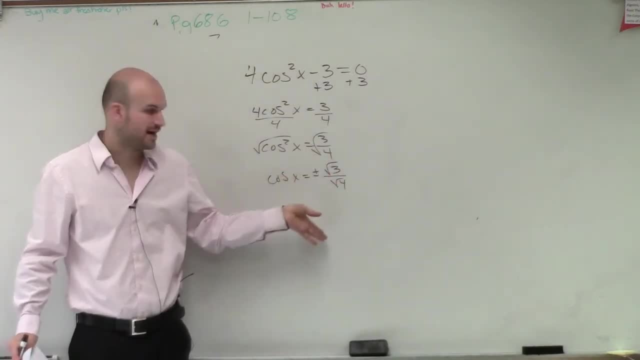 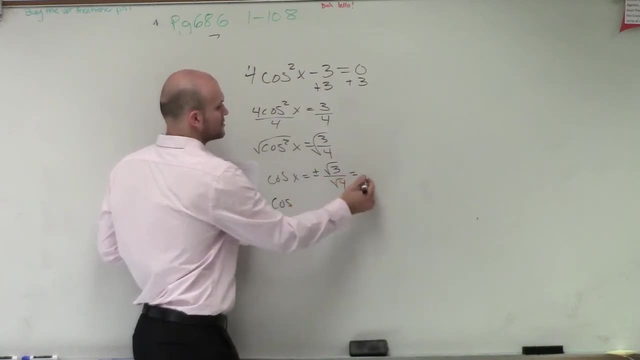 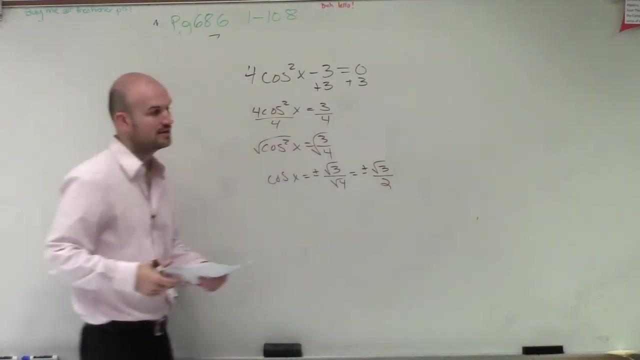 I can distribute that square root to just the top and the bottom. Therefore, I know that this is going to be just 2, right? So actually I'll just say so: square root equals plus the square root of 3 over 2.. So what they're asking us to do is find the values when cosine. 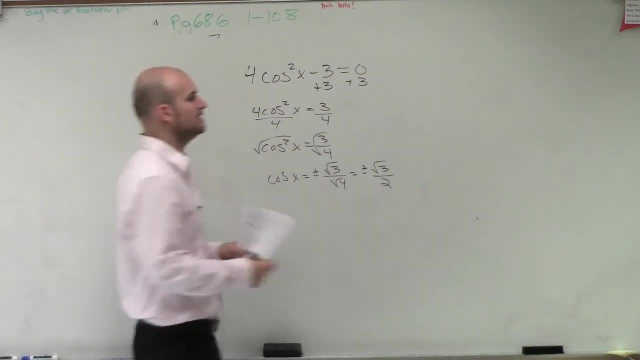 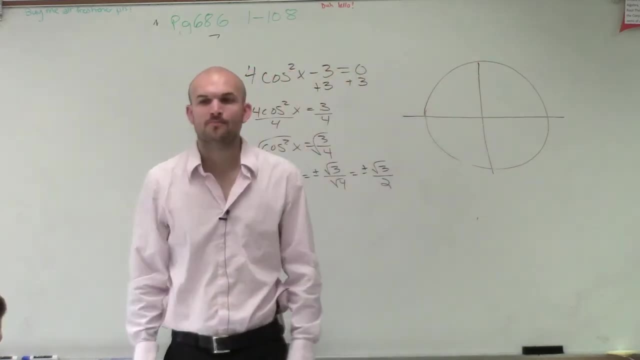 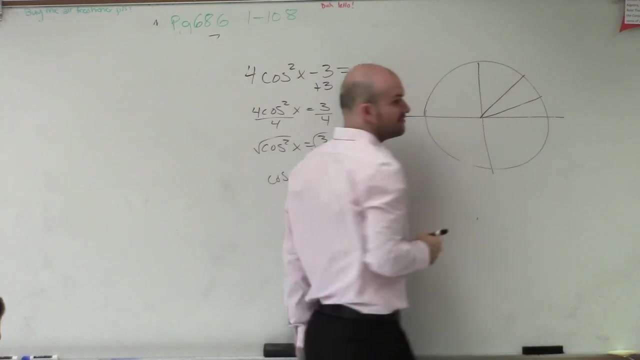 of x is equal to plus or minus the square root of 3 over 2.. So we need to go back and remember: when is the cosine value equal to that? Now let's just go back and remember our major points. We had the first one, which is 30 degrees or pi over 6.. We had 45 degrees. 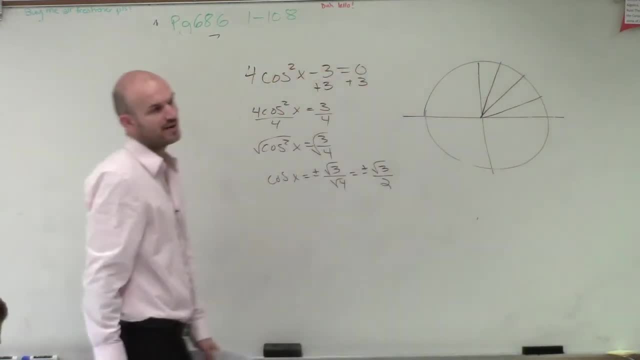 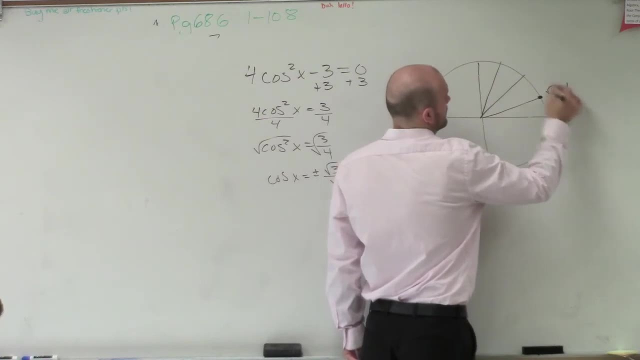 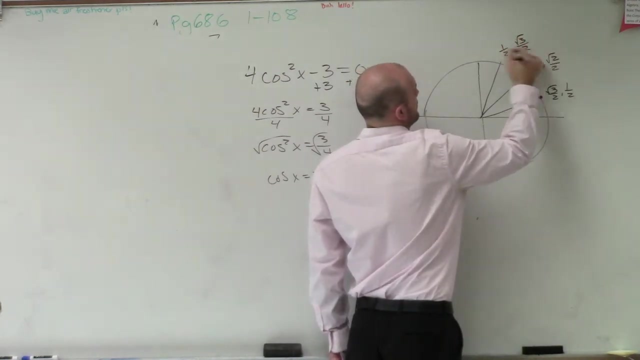 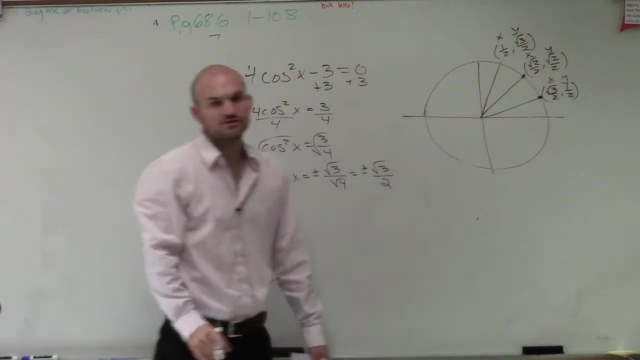 or pi over 4.. And then we had 60 degrees, which would be pi over 3.. So I'll write the coordinate points, if you guys forgot them, And remember these are all x, y, xy. So out of those three points, when is cosine squared? 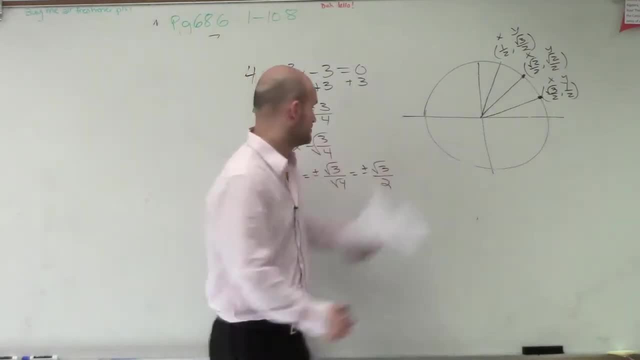 of 3 over 2? At pi over 6, right, So we could say x equals pi over 6.. And then remember, when else would cosine of x equal pi over 6?? Right, it's going to be this point, right. 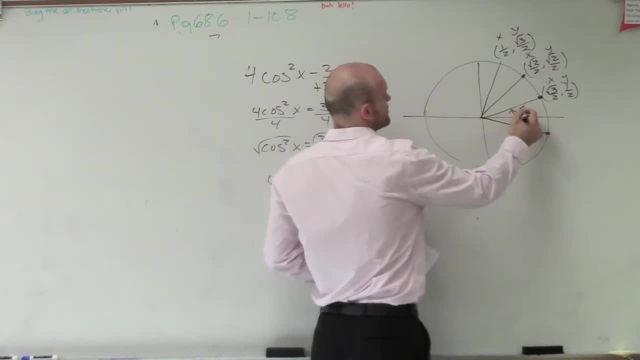 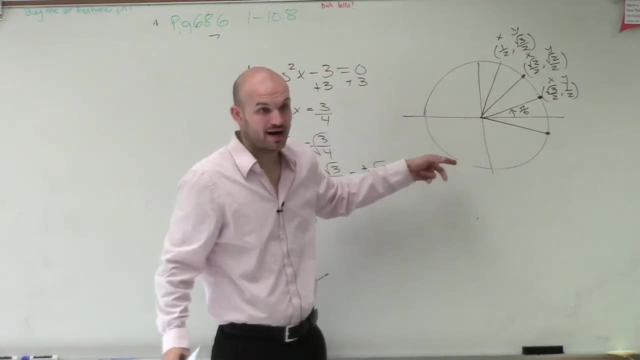 down here, right And then so if you know that this is pi over 6, this is pi away, right? This is going to be pi away from 2 pi. Remember, all the way around the circle is 2 pi, right? 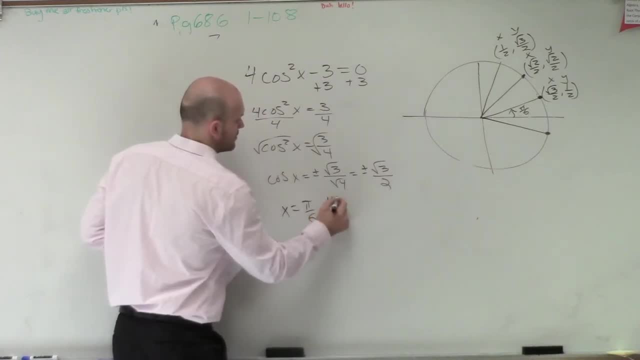 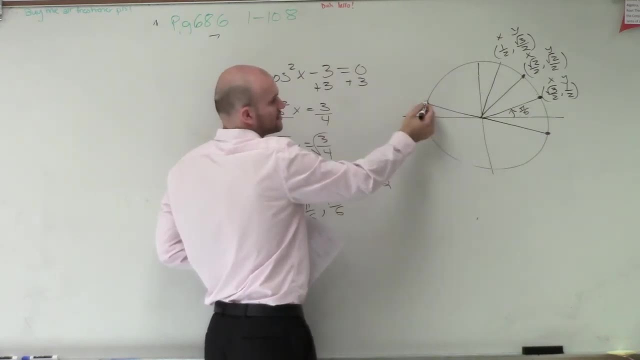 So it would be 11 pi over 6, right, Because 5 pi over 6 would be over here. right, Because it would be 6 pi over 6.. So 11 pi over 6 over here, which would be a negative square root. 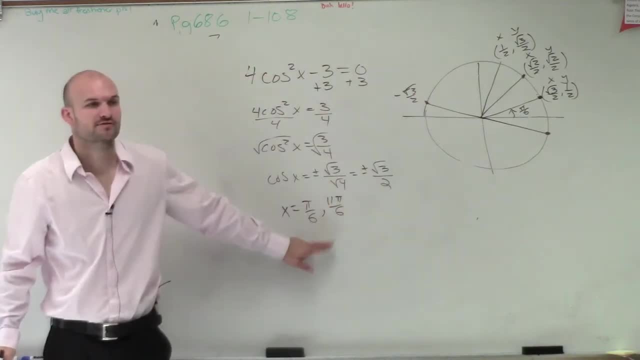 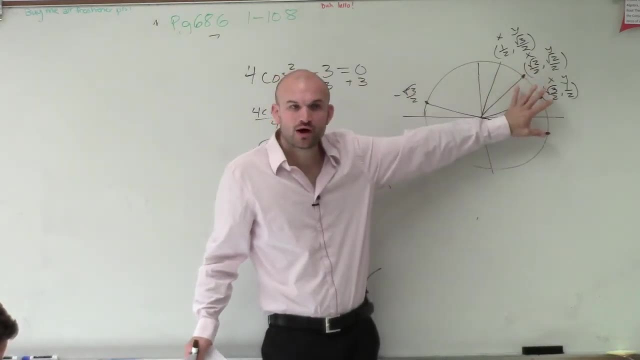 of 3 pi over 2.. But we're just looking for the positive value, so it would be 11 pi over 6.. Got it? So you guys have to remember, if anything, just remember these first three quadrants, these third coordinates, because then you can relate them. Yes, What? 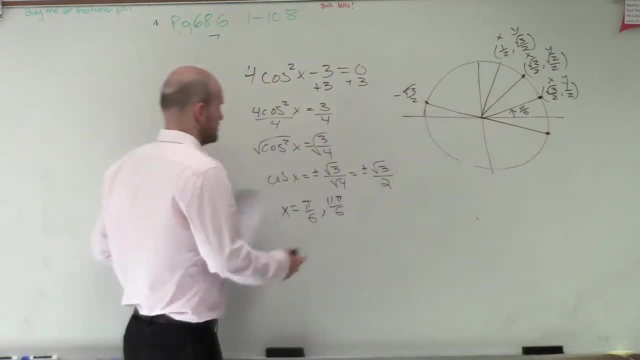 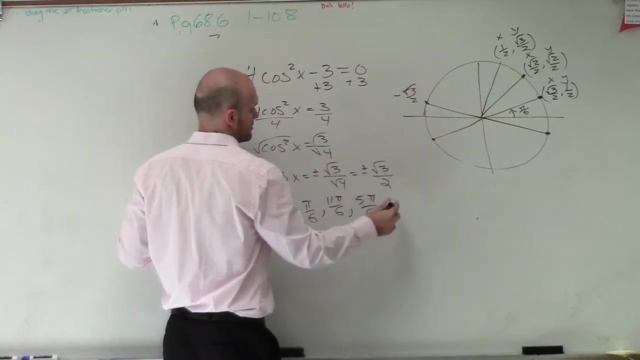 Oh, you're right. actually I'm sorry, You're right, it is plus or minus right, So we need to do the negatives as well. So, yes, 5 over 6 works as well. Sorry, So 5 over 6, and then this point right here, which would be 7 pi over 6.. And do they give?